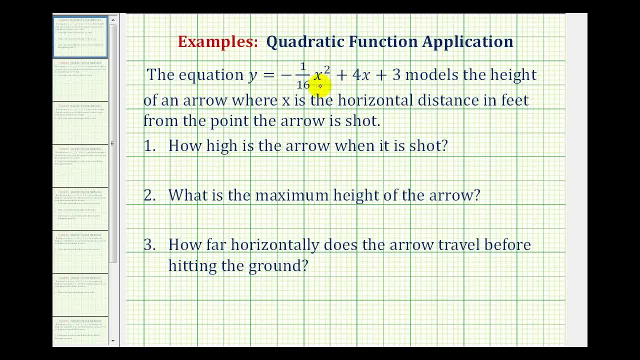 The equation y equals negative 1, 16th x squared plus 4x plus 3 models the height of an arrow, where x is the horizontal distance in feet from the point the arrow is shot. So y represents the height in feet and x represents the horizontal distance traveled in feet. 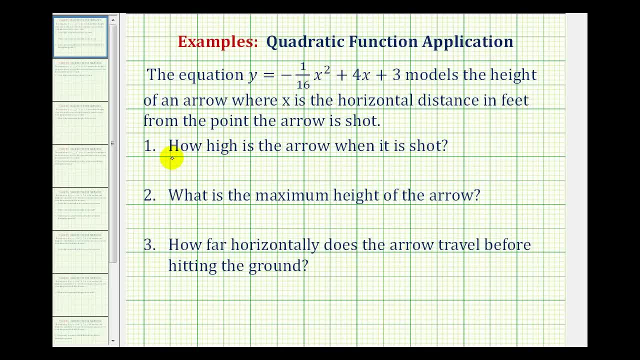 We want to answer the following three questions. Number one: how high is the arrow when it is shot? Number two: what is the maximum height of the arrow? And number three: how far horizontally does the arrow travel before hitting the ground? So let's go through these one at a time. 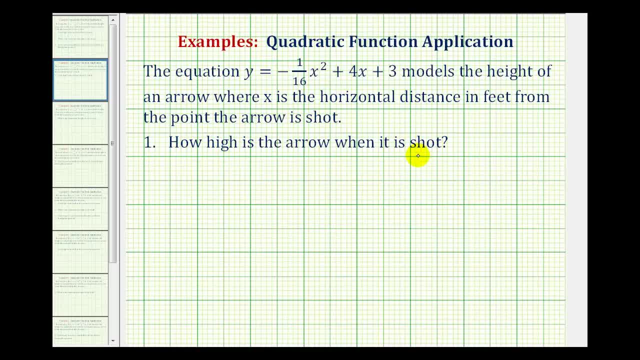 To answer the first question of how high the arrow is when it is shot, right at the instant the arrow is shot, the arrow has not traveled horizontally. Therefore, to answer this question, we're going to set x equal to 0 and then solve for y. 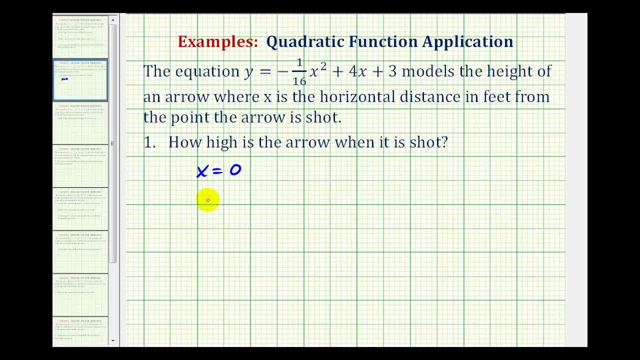 So if we let x equal 0,, we want to evaluate y of 0. Which would be negative: 1 16th times 0, squared plus 4 times 0 plus 3.. So y of 0 is just going to be 0 plus 0 plus 3 or 3.. 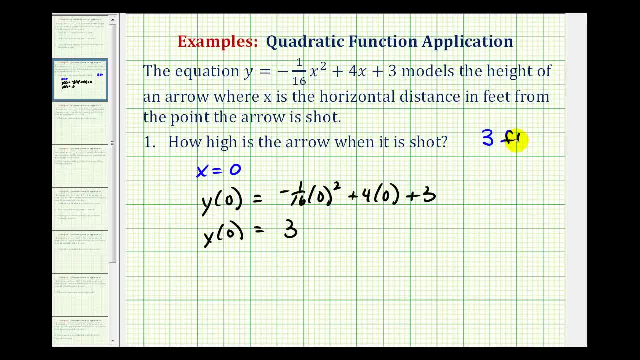 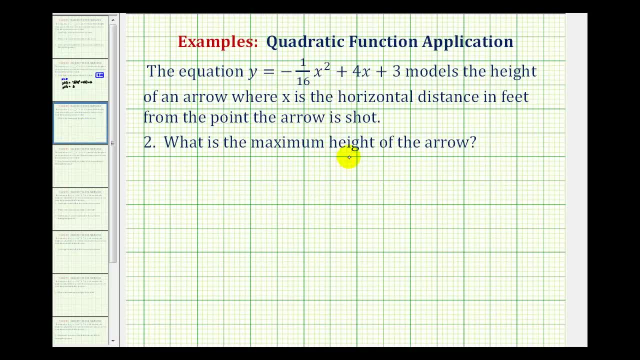 Therefore, the arrow starts at a height of 3 feet. Number two: we want to determine the maximum height of the arrow. Notice: our equation is a. We're going to use the quadratic equation and therefore the graph is a parabola. 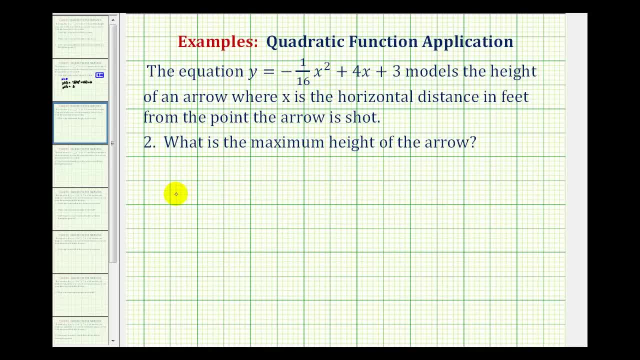 And because a is negative. it's a parabola that opens down or looks something like this: So the maximum height of the arrow would be represented by the vertex. So we'll find the vertex where the x coordinate will represent the horizontal distance traveled. 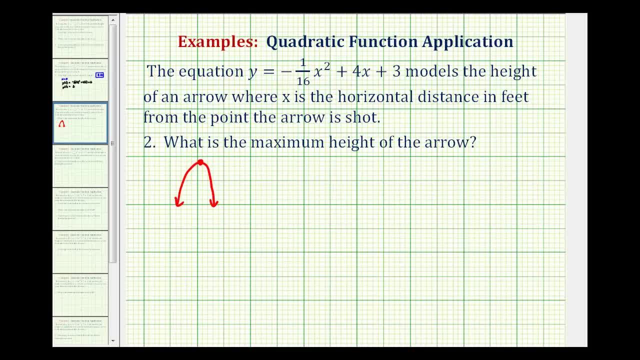 and the y coordinate will be the maximum height. Remember, the coordinates of the vertex are negative b over 2a, comma f of negative b over 2a. So we'll start by determining the x coordinate of the vertex using this formula here. 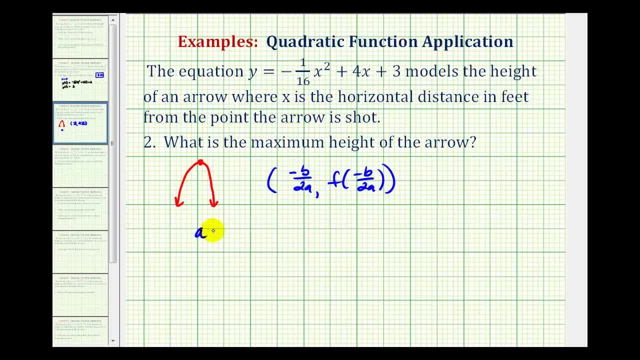 Notice: a is equal to negative 1 16th. b is equal to positive 4, and we don't need c, but c is equal to 3.. So the x coordinate is going to be equal to negative b or negative 4 divided by 2 times a or 2 times negative 1 16th. 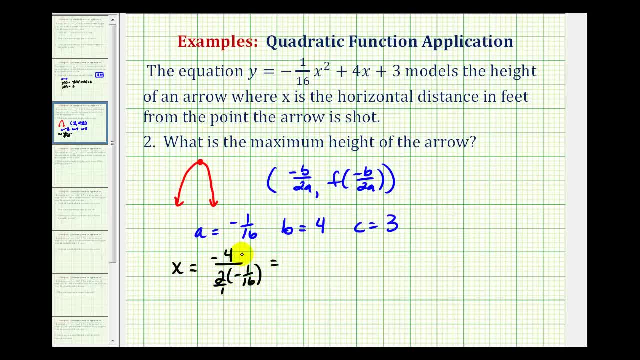 So let's put this 2 over 1.. We're going to have negative 4 divided by the 2 and the 16. simplify This simplifies to 1.. This simplifies to 8.. So we have negative 1- 8th. 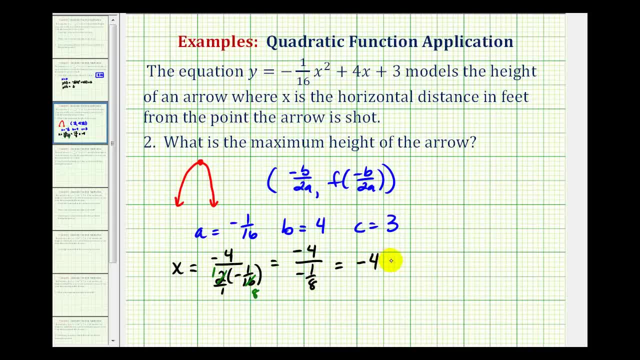 So we'll have negative 4 times a. So we'll have negative 1- 8th. So we'll have negative 4 times a, The reciprocal of negative 1- 8th, which is just negative 8 or negative 8 over 1.. 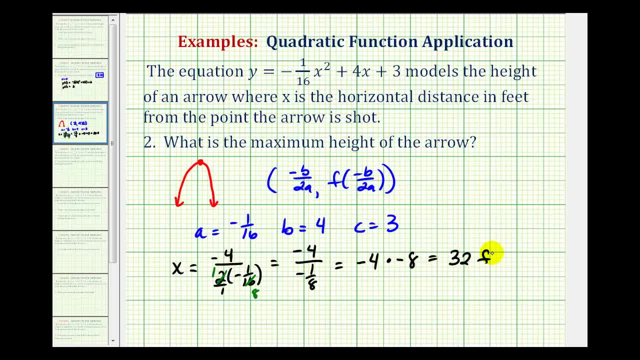 So x is equal to 32 or 32 feet. Again, this is the horizontal distance traveled at the maximum height. So to find the maximum height we'll now have to substitute x equals 32 back into the original equation. So we want to find y of 32, which is going to be equal to negative 1 16th times 32 squared. 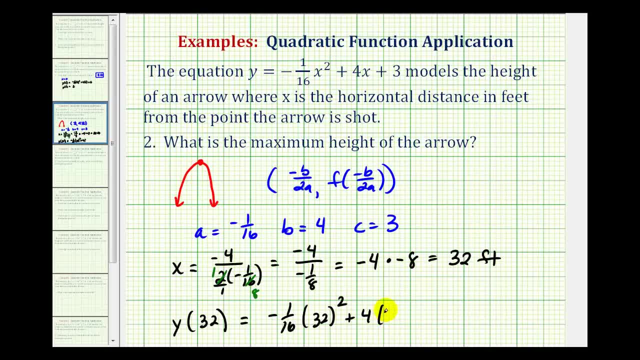 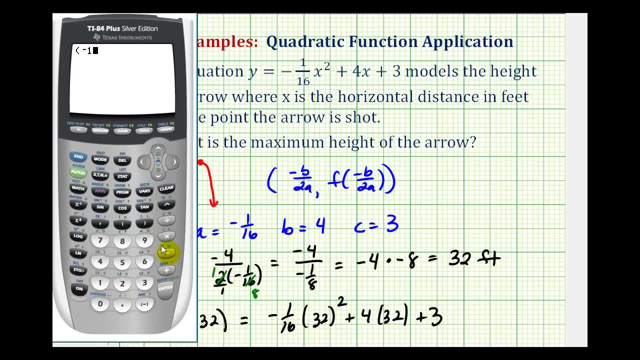 plus 4 times 32, plus 3.. Let's evaluate this on the calculator. So we have negative 1 16th times 32, squared plus 4 times 32, plus 3.. So the maximum height is equal to 62.. 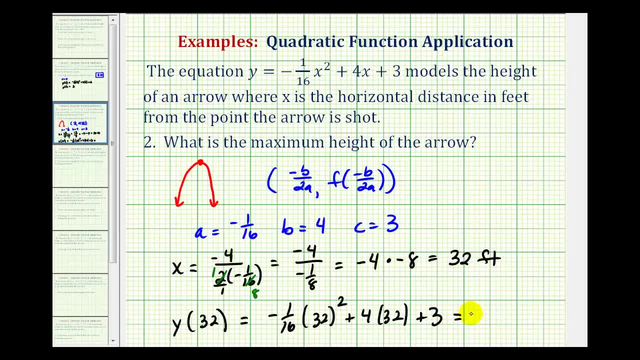 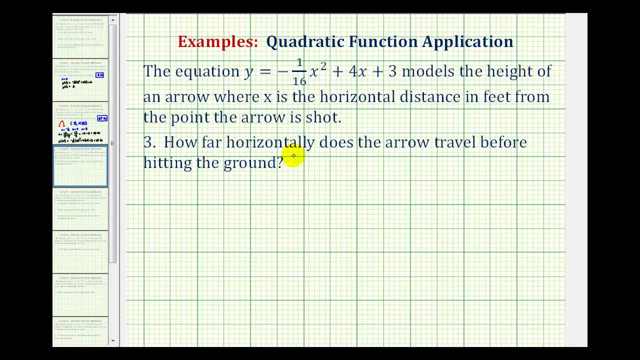 So this is going to be equal to 67 feet. And then for the third question, we want to determine how far horizontally does the arrow travel before hitting the ground. Well, when the arrow hits the ground, the vertical height would be 0, which means y would be equal to 0.. 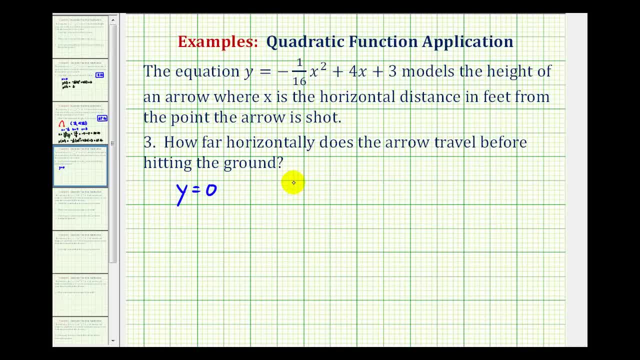 So we're going to set y equal to 0.. So we'd have the equation: zero equals negative one-sixteenth x squared plus four, x plus three. Now this equation is not going to factor, so we'll have to solve this using the quadratic formula. 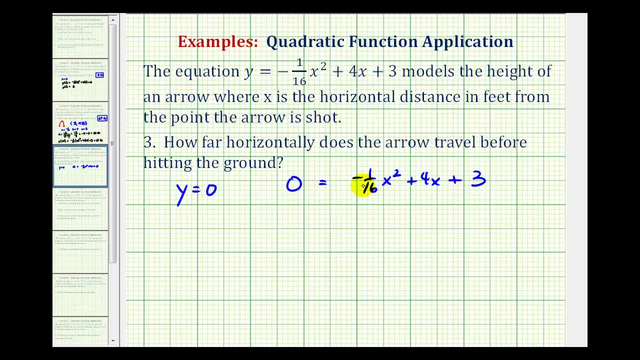 And it's going to be easier if we eliminate this fraction by multiplying both sides by 16. or if we want a to be positive, let's multiply both sides by negative 16.. Remember, multiplying both sides of an equation by a constant is not going to change the solutions. 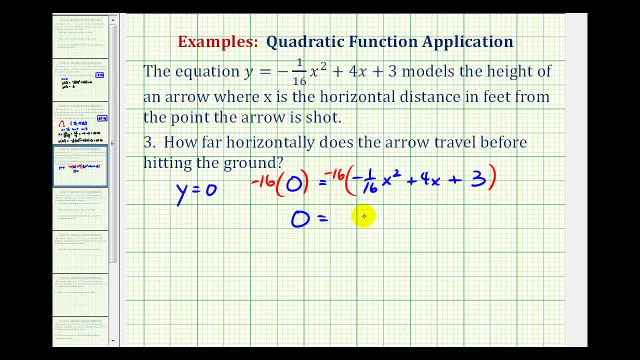 So we'll have zero equals. this would be positive one x squared minus 64 x, and this would be minus 48.. So now we'll use the quadratic formula where a is equal to one, b is equal to negative 64 and c is equal to negative 64. 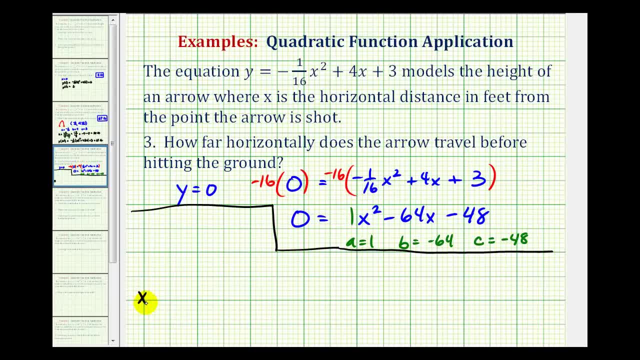 So we'll have x equals negative b or negative 64. that will be positive 64 plus or minus the square root of b squared, which is negative, 64 squared minus four times a, which is one times c, which is negative, 48, all over two times a, or two times one, which is two. 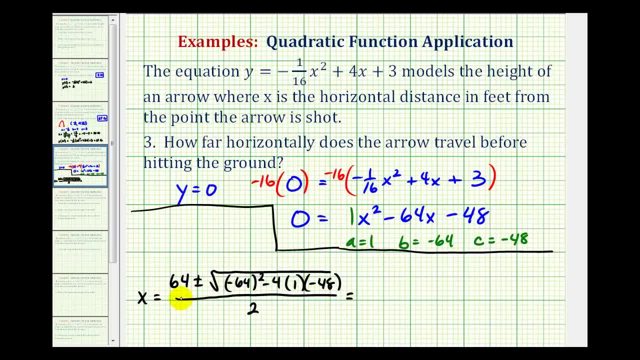 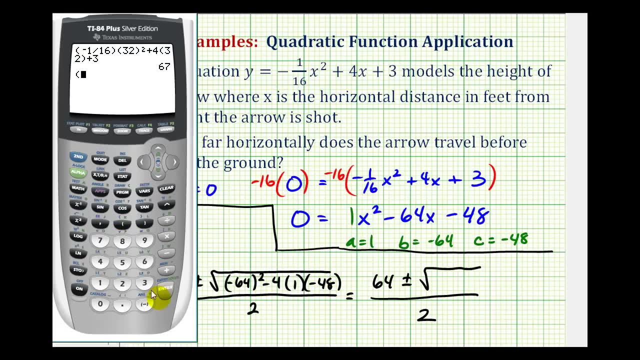 So now let's go ahead and begin to simplify this. We'll have: x equals 64 plus or minus. we'll come back to the discriminant. all this is divided by two. Let's evaluate this on the calculator. So the discriminant is negative: 64 squared minus four times one, which we don't need. 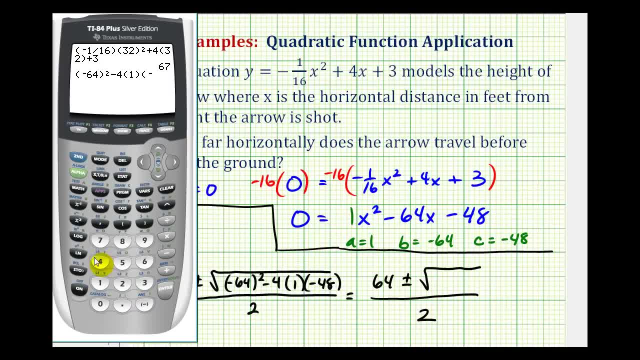 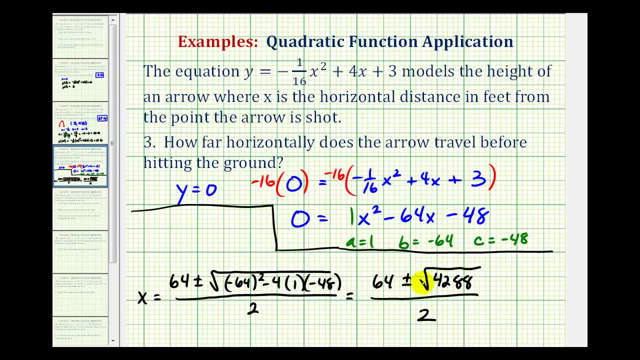 but I'll put it in there- times negative 48. So we have 4,288 underneath the square root and because we know x has to be positive- it's a horizontal distance- we only have to be concerned about the positive solution here, which would be 64 plus the square root of 4,288, all divided by two. 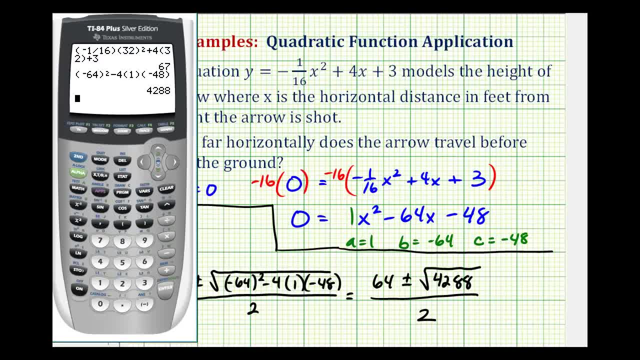 So let's go back to the calculator. Our numerator is going to be 64 plus 4288.. So we have: x equals negative 64 squared minus one, plus the square root of four thousand two hundred eighty-eight. Notice how we have two closed parentheses here, one for the square root and one for the numerator. 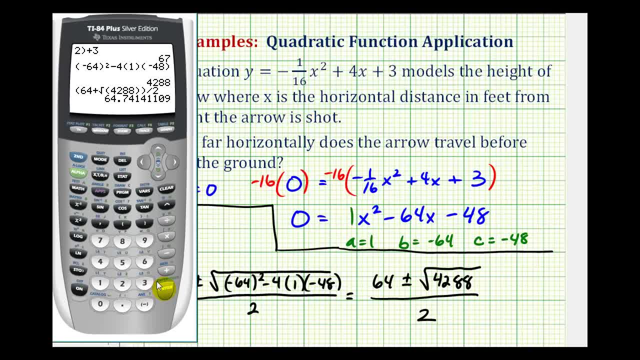 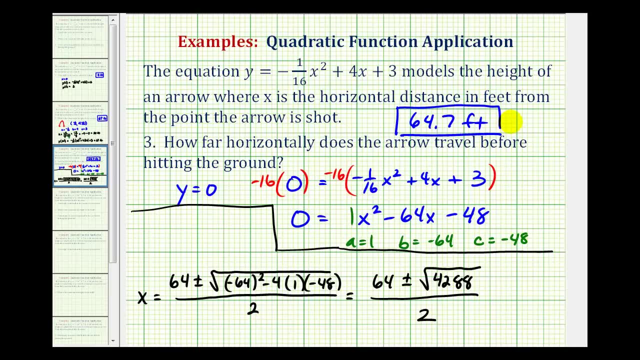 divided by two, So the arrow travels approximately sixty-four point seven feet horizontally before hitting the ground. Okay, I hope this example helps. 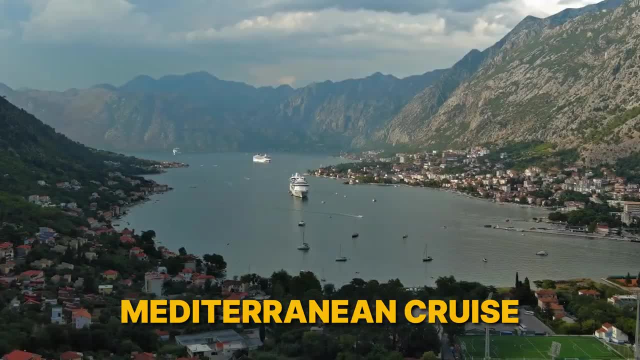 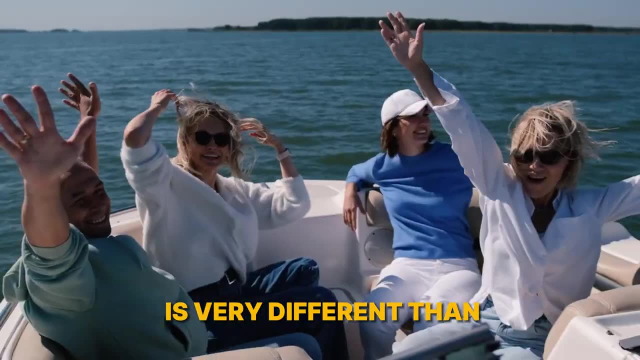 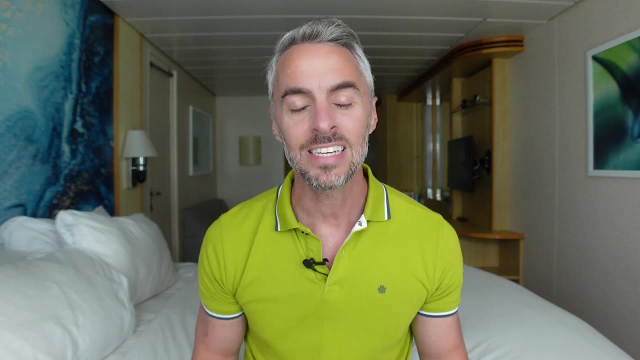 Are you tired of sailing around the Caribbean and looking at doing your first Mediterranean cruise? to spice things up a little bit, You want to pay attention to this video on eight ways that a Mediterranean cruise is very different than a Caribbean cruise. Hey everybody, it's Brandon The Weekend Cruiser, where I go on a weekend cruise just about every weekend. 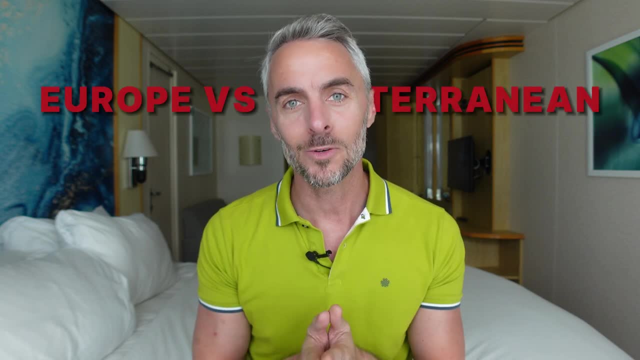 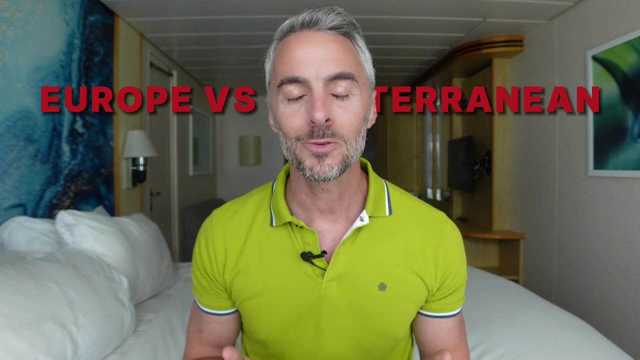 But I also love getting out of the Caribbean and seeing the rest of the world via cruise ship, And so I wanted to make this video. if you're looking at making the jump over the pond to check out a Mediterranean cruise, what you can expect- There are eight things here that 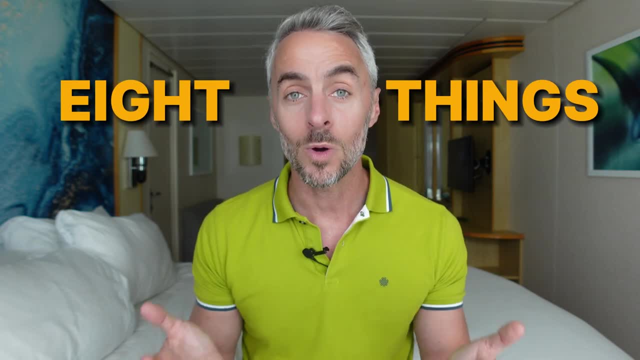 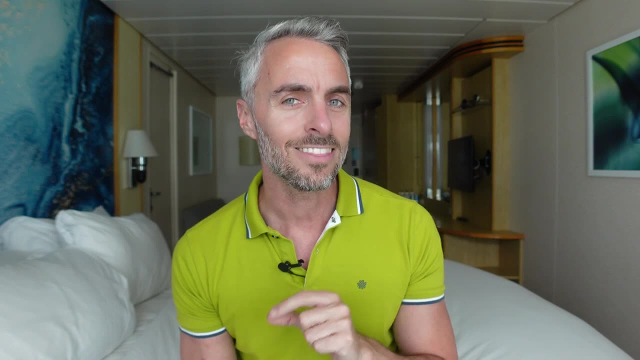 I'm going to go through in pretty quick order, but I hope that this will help you prepare for your Mediterranean sailing. The first thing that you're going to notice here is: if you go on a seven-night sailing, what's the one night that you really look forward to in the main dining room? 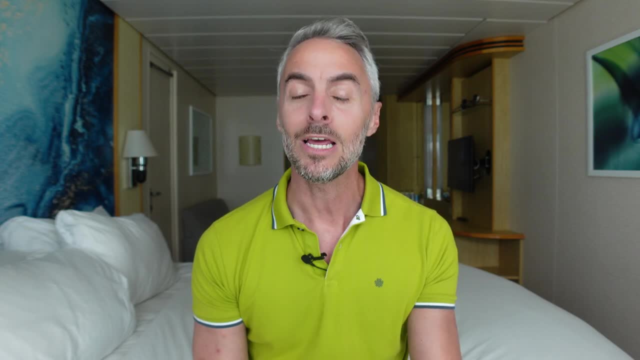 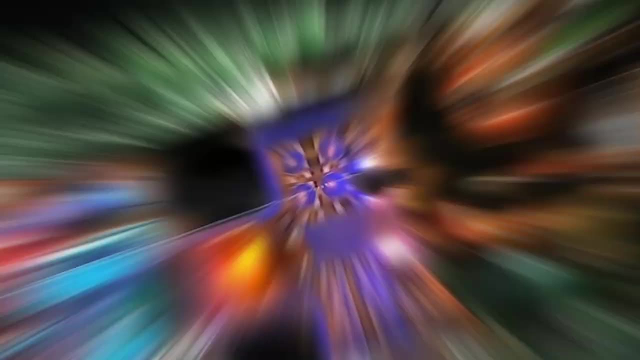 Formal night. That is absolutely correct. And why do we look forward to formal night? Because we get lobster, And that is the awesome part to formal night. However, over in the Mediterranean you're not going to have two formal nights like you do in the Caribbean. 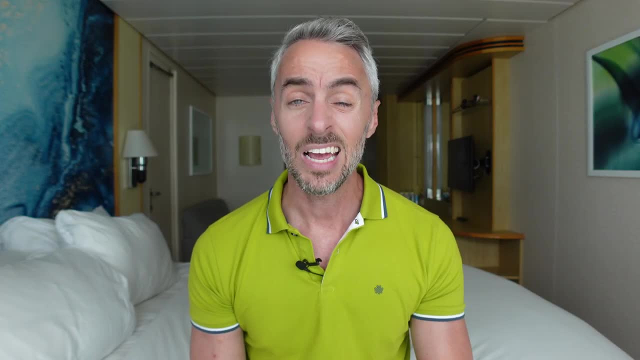 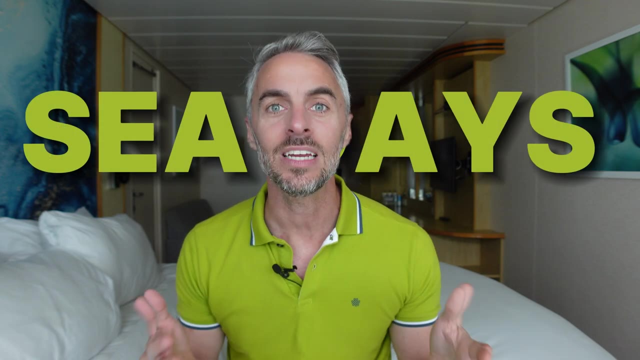 You're going to have one formal night and that one formal night it's not going to come with lobster. The second thing that you're going to notice is that in the Caribbean you're going to have two or three sea days where you can enjoy the ship If you're going over to Europe, into the Mediterranean. they think that you're going to actually see Europe and Mediterranean, which is normally the case, And so you're not going to have very many sea days. You'll be lucky if you get one. I've been on one cruise that had a port every single day. It is exhausting, So you're going. 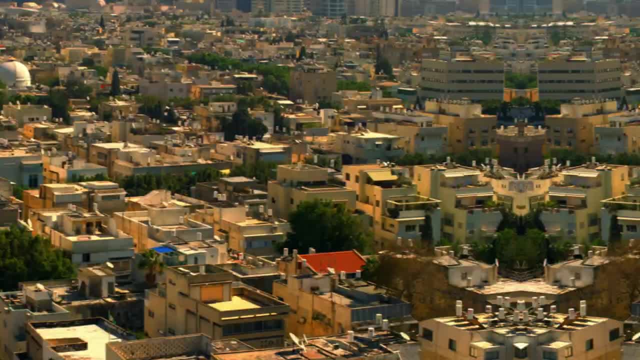 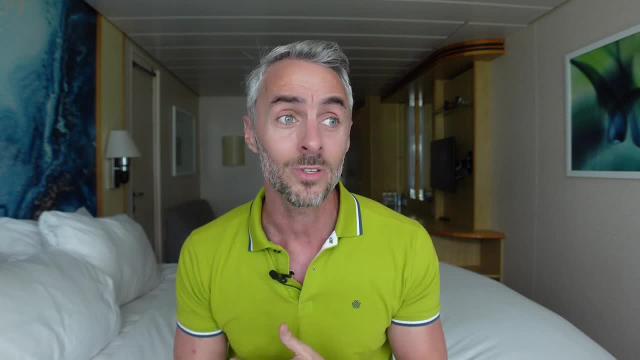 to need to make sure that you're going with a ton of energy for this sailing, So that you can go explore a new country, a new city, every single day that you are on your cruise. Even on one of my last cruises, it had a port every day I didn't get off. the last day I made a sea. over to Europe. If you are in the Caribbean, you can find excursions for $30, $50, $75. That is not going to be the case over in Europe. You're looking at paying a minimum of probably $125, $150, and you can go up to $500. Most of mine- I think I was averaging around $200 to $225. 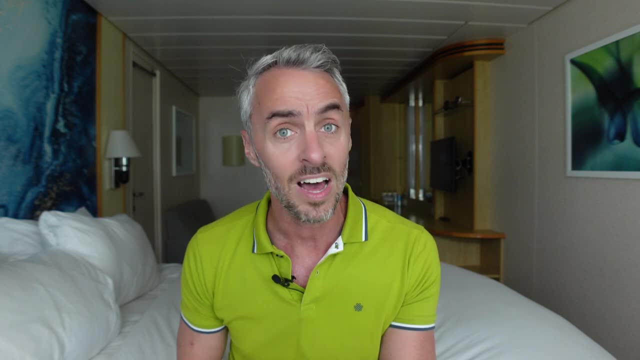 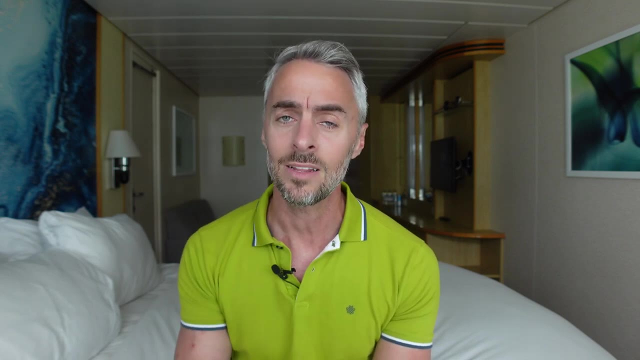 per excursion per person, And if you were doing this for five or six days, that's going to add up really, really quick. And one of the downsides of going over to the Mediterranean is a lot of these ports aren't equipped to handle cruise ships. They've got.